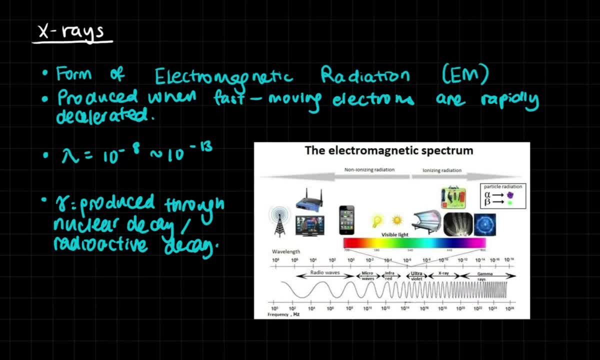 gamma rays that have exactly the same wavelength, which means we need to define x-rays and gamma rays in order to be able to differentiate them from each other, because we can't do that solely depending on their wavelengths. So the definition of an x-ray is a form of 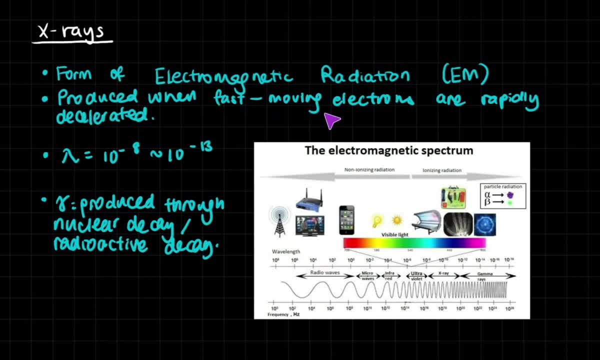 electromagnetic radiation that is produced when fast-moving electrons are rapidly decelerated. So when electrons are extremely quickly moving and something will make them stop or make them change course, they go through very rapid deceleration and that basically creates an x-ray. The electrons are moving in the form of a wave instead of like a straight line, so as they 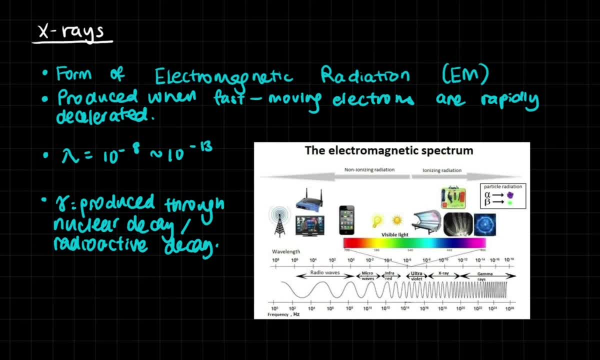 kind of decelerate the shift in their electric field, will create a shift in their magnetic field, and it would then create another shift in the electric field, and then so on and so on and so forth, until there is an actual photon that is produced. So that is how x-rays are produced, and 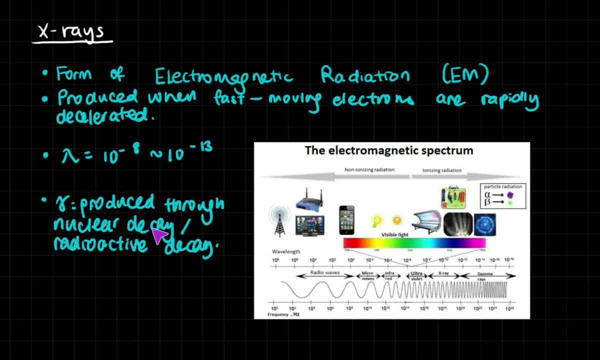 on the contrary, gamma rays are produced through nuclear decay or radioactive decay, which you may already know if you've studied x-rays. So that's how x-rays are produced and, on the contrary, any form of nuclear physics. There are three main types of radiation for nuclear physics. 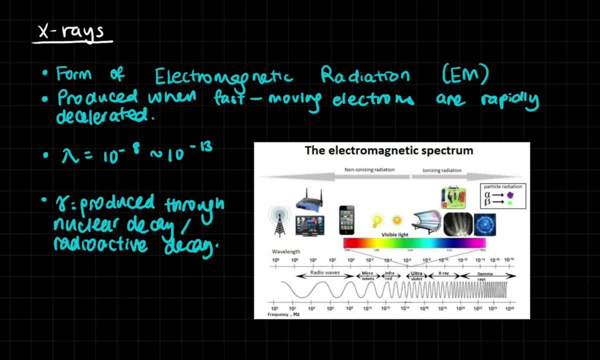 There is alpha radiation and there's beta radiation and there's also gamma radiation. Alpha radiation and beta radiation are matter. They're matter and they basically get released to stabilize a nucleus and during these radiations there could be an excited state for the nucleus. 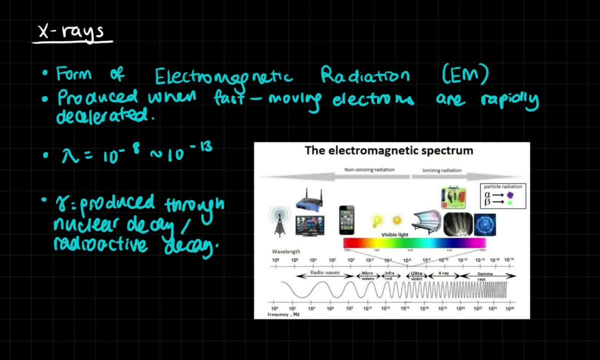 where it is unstable, and so they let out a bit of energy in the form of a gamma ray, which is not matter, it's an electromagnetic wave- in order to further stabilize itself. So that is the difference between an x-ray and a gamma ray. It's just. you have to define it in terms of the method of their production. 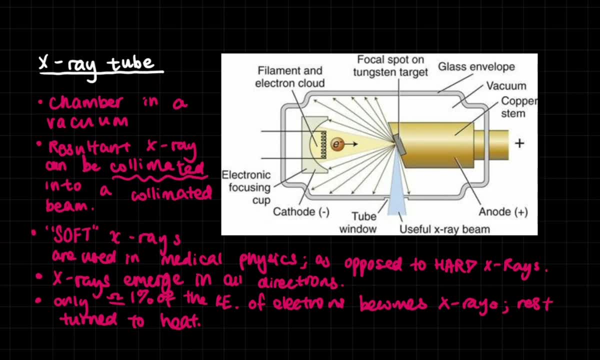 So what we're really trying to do with x-ray production is: x-rays are used to scan our bodies in medical physics and they can allow us to see right through them and see our bones and our innards and everything. In order for us to use these things, we need to be able to see our bones. 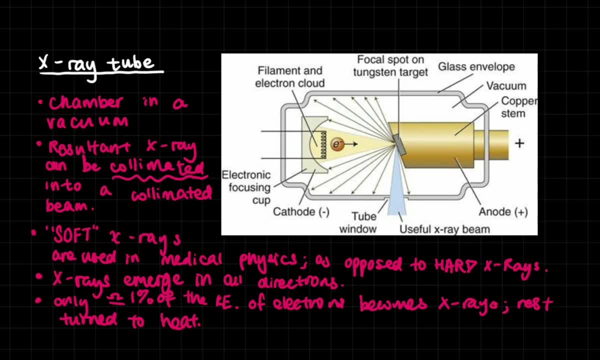 and we need to find a way to produce these x-rays on demand just by flipping on a switch. So for that we have an x-ray tube. So this x-ray tube will allow us to produce the x-rays. Just from the definition of the x-rays, you already know how x-rays are made. 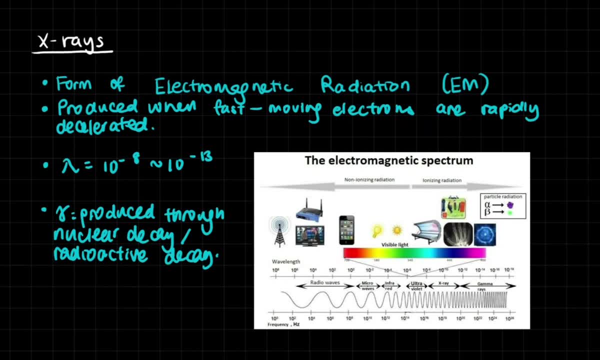 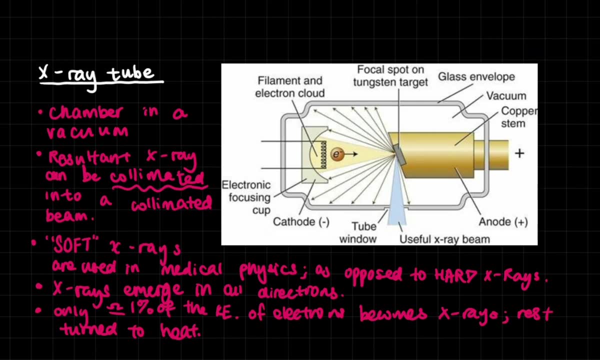 You know that you need fast moving electrons and they have to be rapidly decelerated. So, ultimately, with this device, we're trying to do three things. First of all, we're trying to mix the electrons that are very fast moving. Second of all, we're trying to decelerate. 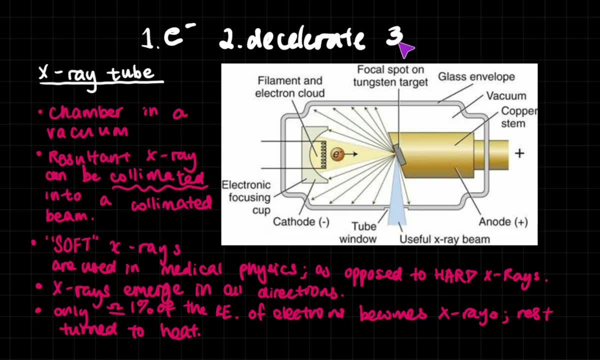 these electrons very quickly, very rapidly. And third of all, we want to collect the x-rays that are produced. So we have to fulfill these three things using our device, And this device is called an x-ray tube, which we're going to talk about right now. So this is what an x-ray tube looks. 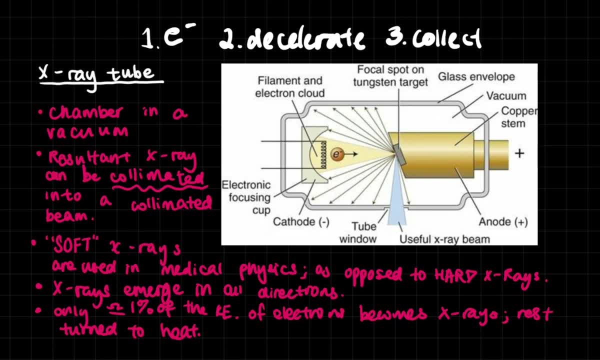 like, And just on the get-go, I'm going to point out some parts of the x-ray tube. So here is the cathode and over here you have like a filament and it's a negative terminal over here. so you would have you know you have a positive sign over here. 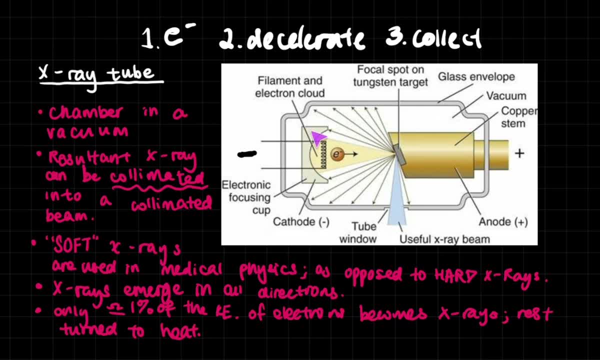 and you would have a negative sign over here. so this is a cathode. it's negative charge and there's a positive anode over here. what that creates is it creates because there's positive charge here and negative charge here. that creates an electric field throughout this chamber. so if there was an electron, it would. 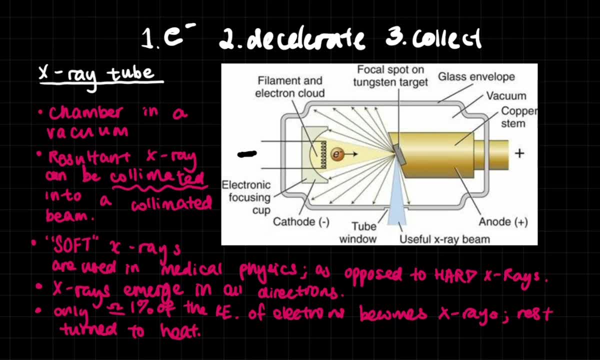 move in this direction due to the electric field. so as the electrons are released, they are actually accelerated towards the positive side, because there is a force on the electron due to the electric field and we know that F equals ma, so this will basically create an acceleration, which is a, so they will be 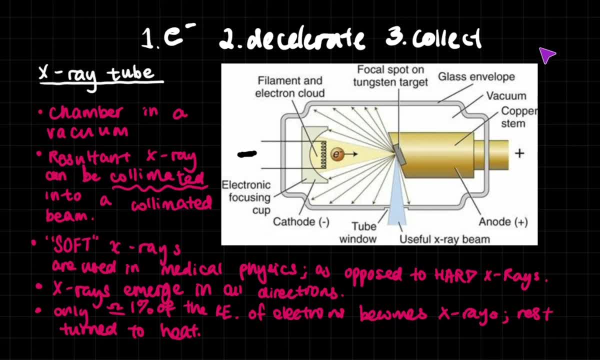 made to move very quickly. so we've already fulfilled one of our three requirements with just to have fast-moving electrons. now let's talk about the deceleration when the fast-moving electrons hit this certain target. and this target is in the anode. it's a tungsten target, it's a type of metal, and when they hit it, 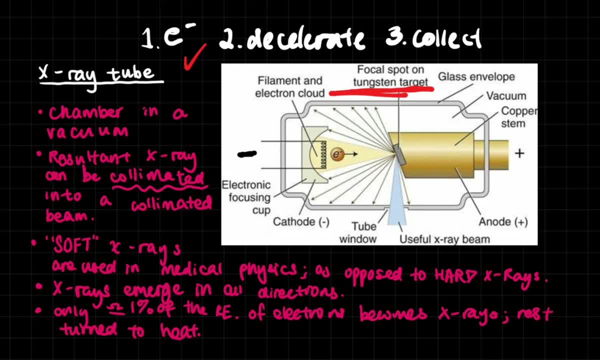 they're going to be made to stop, obviously. and the motion of stopping imagine, if you kind of like zoom in through time and you look at the electron in extremely slow motion. they are basically decelerating at a very quick rate and so as they hit this, they do celebrate rapidly. so we know that. 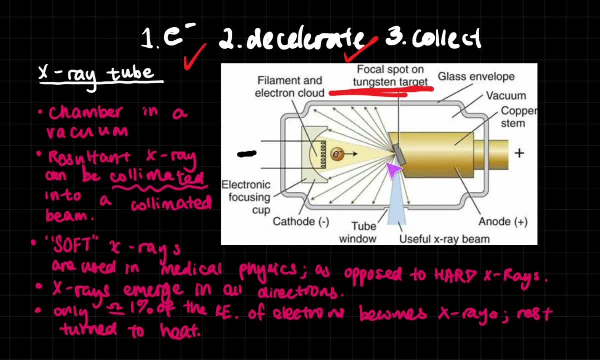 happens and finally, we are going to have x-rays that are spread through this deceleration in all directions, and we need to collect the array, and so there's a tiny window over here in the chamber and this is where the x-ray will come out, and it's a useful x-ray beam. so what we actually do is we have a 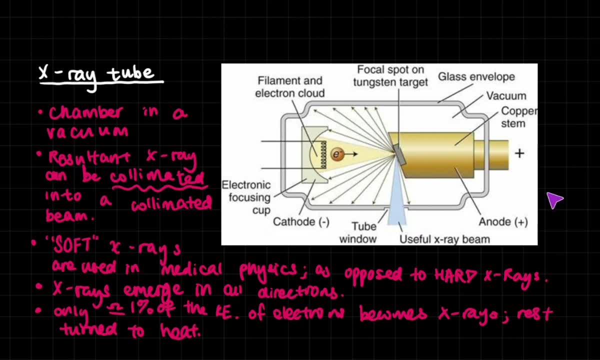 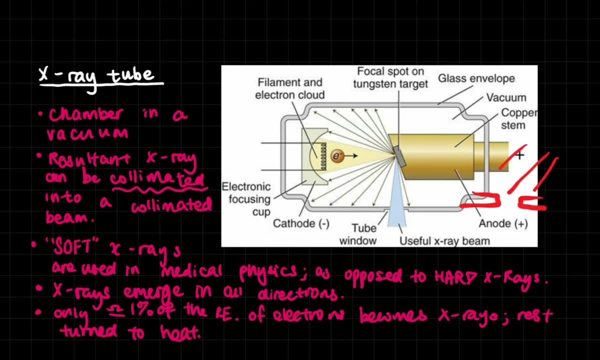 we have the walls over here and the walls kind of look like this and the x-rays are going to basically hit and only those that go through this wall is going to come out. so eventually you have a parallel x-ray. this parallel ray is very important because we want something. 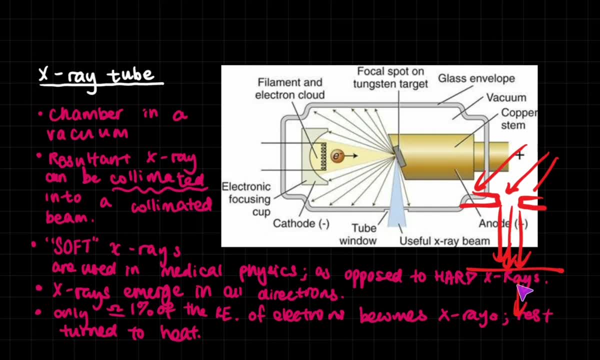 that is even so. when we put it through skin it's going to give us like an even concentration or intensity of x-ray on the other side of this. if we had, like, a rays going to one side, it would not give us a fair image of what's actually inside of the skin. so we need parallel rays. we can't have rays that are 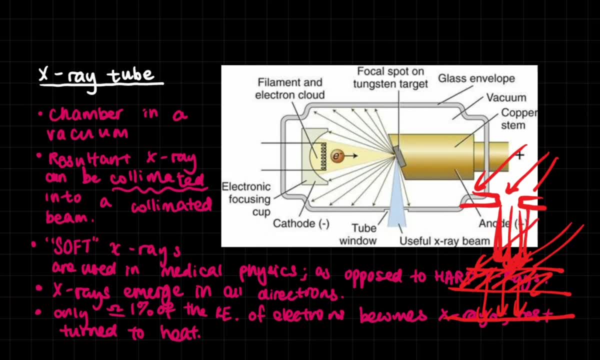 going in all sorts of directions. so this parallel ray is what is called a collimated, a collimated beam, and the process of making it parallel is collimation, the process of collimation. so that's essentially what happens. you have the acceleration, you have the deceleration, and then 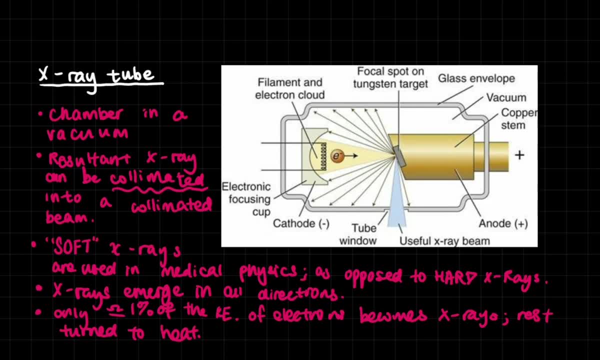 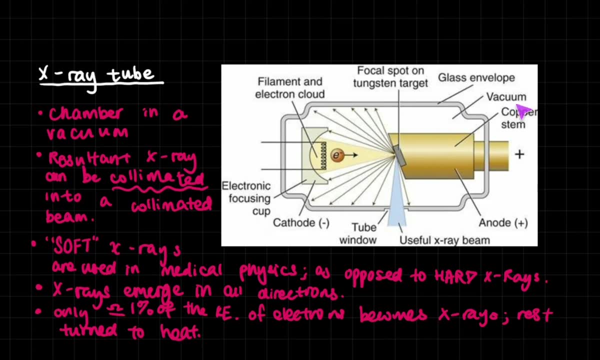 you have the collection of a useful x-ray beam. now let's go into a little bit more detail about the various parts of this x-ray tube. so this chamber is actually in a vacuum. as you can see, it's a vacuum inside here, and the reason why we need to have a vacuum inside of this chamber is 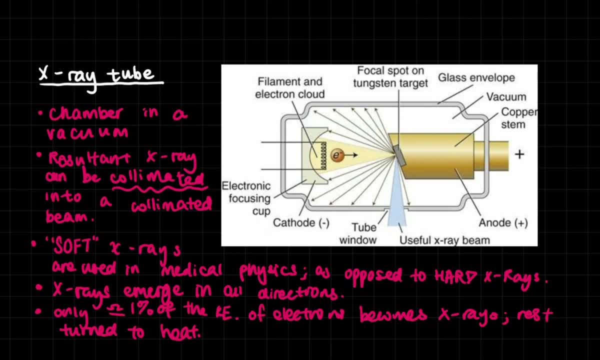 because if it was paired, it was filled with air molecules, then the motion of the electrons would be basically, the air molecules would impede the the. the air molecules would impede the motion of the x-rays. They would collide with the air molecules and they would 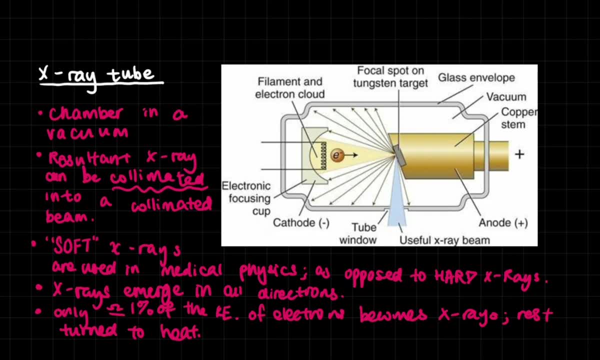 not make it to the end of their path and to the tungsten target, So they would be scattered everywhere and so you wouldn't actually get all the x-rays that you could get, which is why we need to put it in a vacuum to have a clear. 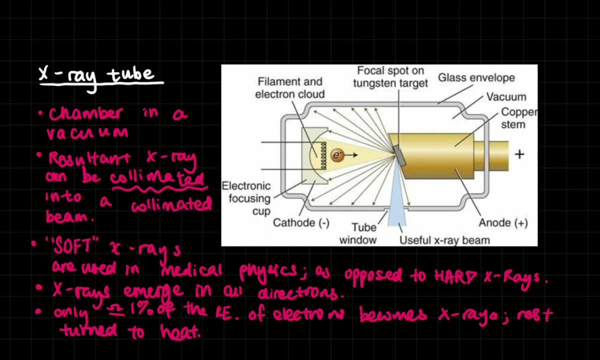 path for the electrons. Secondly, we've already talked about the collimation. The resultant x-ray is going to be collimated into a collimated beam. So once we have this useful x-ray beam, we want to use a certain type of x-ray called a. 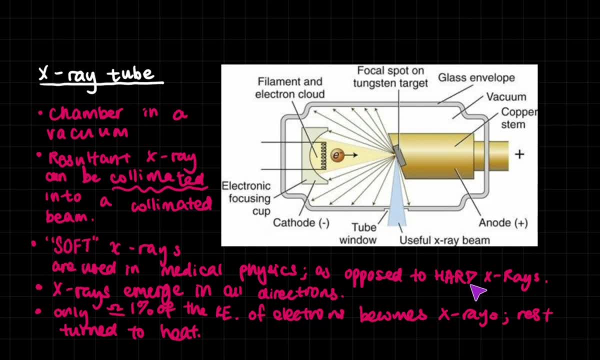 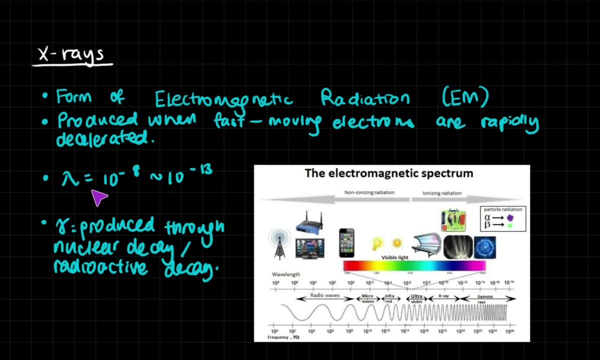 soft x-ray. Soft x-rays, as opposed to hard x-rays, are x-rays that have lower energy. So, as we've looked at previously, we know that the x-rays have a wavelength of in the range of 10 to the power of negative, 8 to the 10 to the 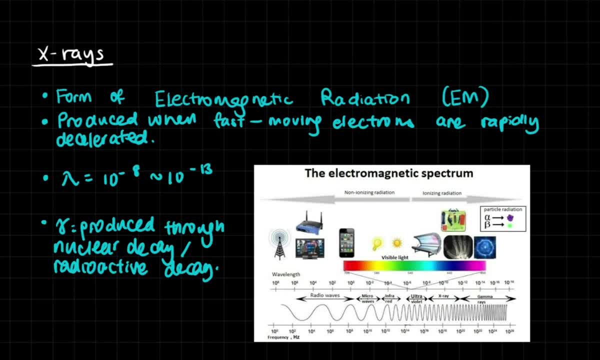 power of negative 13.. If we want lower energy photons, we need to have higher energy wavelength- higher wavelengths for the photons- and that will create a lower frequency. Lower frequency means lower energy, So we're looking at this end of the spectrum here, not this end. So that's the 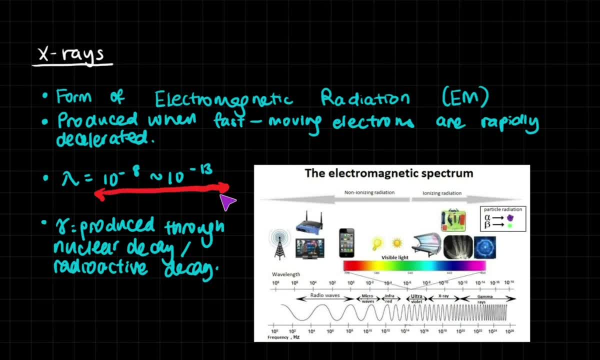 soft electron. So if I could draw like a range over here of wavelengths, this would be soft- Lower energy- And this would be hard, which is higher energy, And we're trying to use the soft energy. The reason for this is because photons 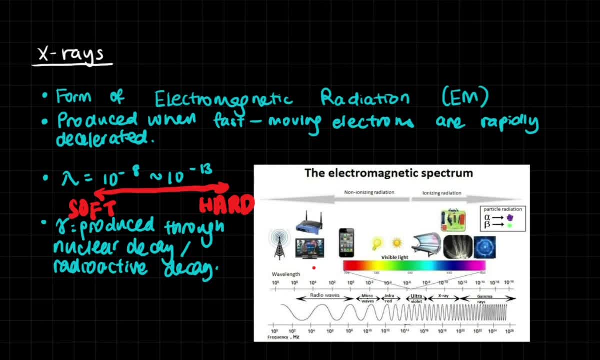 basically can make cells in your body, for instance. they can make it mutate. They can mutate the DNA, for instance, inside your body, and there is a possibility that they can cause health defects when you go under an x-ray And the probability of getting these effects are extremely low because we only use soft 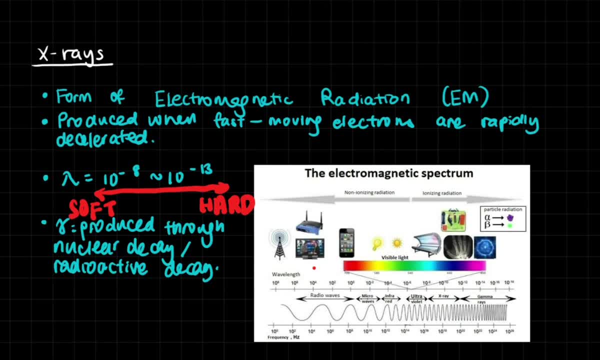 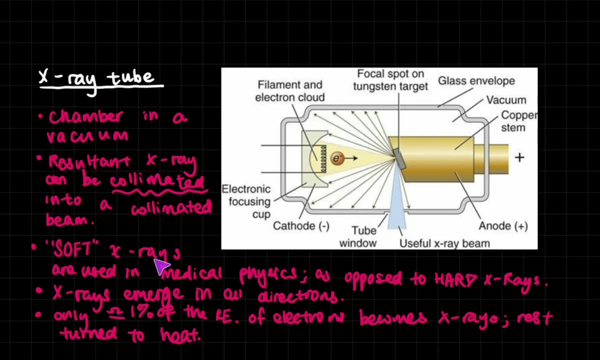 x-rays that have low energy, So it's very unlikely that they're able to produce these kinds of mutations in your skin. As opposed to that, hard x-rays actually kind of overlap into gamma ray territory and they have a much higher probability of causing health defects for you. So that's why we're supposed to use soft x-rays that. 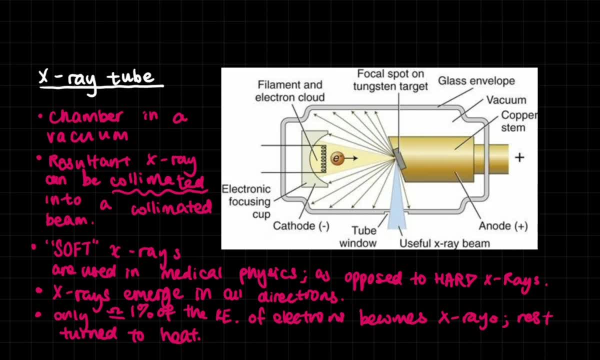 are used in medical physics And the x-rays will emerge in all directions. So what we're essentially doing in terms of energy is we're taking the- obviously we're taking, you know, electrical potential energy. we are converting it into kinetic energy of the 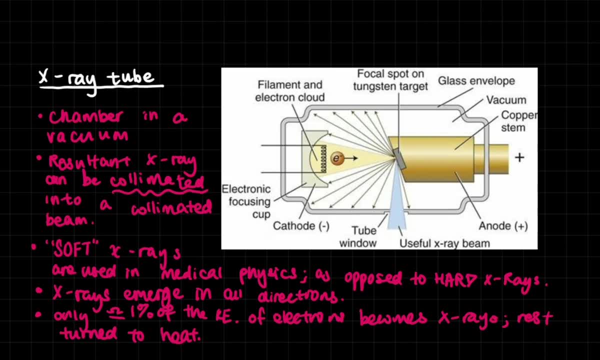 electrons and then we are transforming it into electromagnetic energy in forms of this x-ray. But only 1% of the kinetic energy of the electrons become x-rays and the rest will actually be turned into heat during the rapid deceleration due to friction with, you know, the x-rays. So that's why we're using soft x-rays. 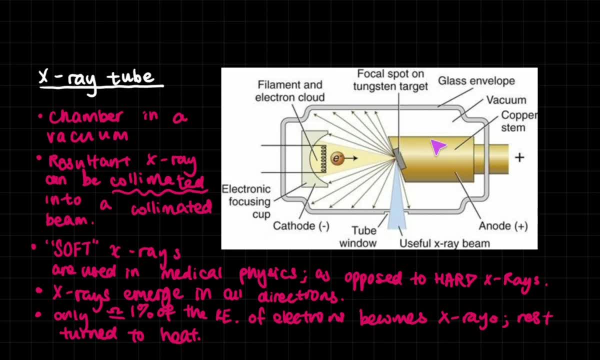 All of the atoms in the metal target and the motion of the electrons and the vibration of it and everything. So most of it turns into heat. but we want that 1% that becomes x-rays and we're trying to collect it. So I think that's about it for the production.